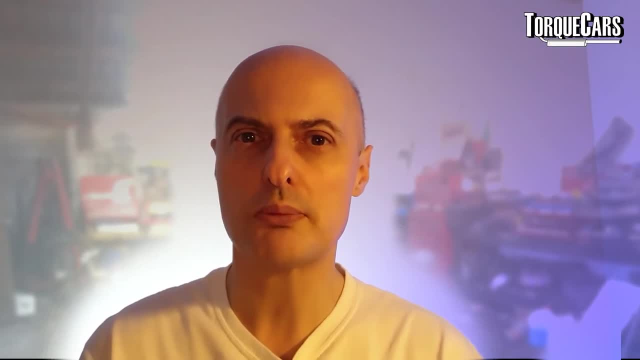 and it's also good for your pocket. If you're conscious of how much fuel you're using, you can keep tabs on your driving style and the types of journeys you make and really stretch out your fuel as far as possible. You do want to save some fuel for the weekend, so driving economically. 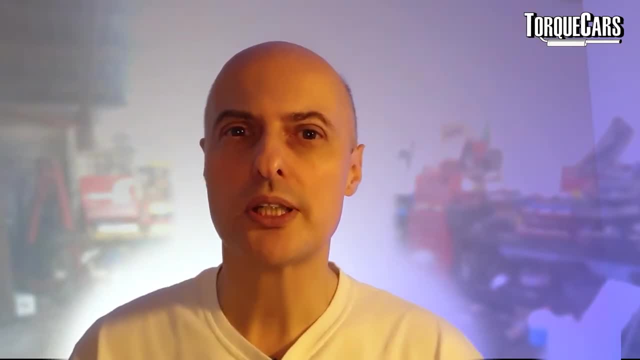 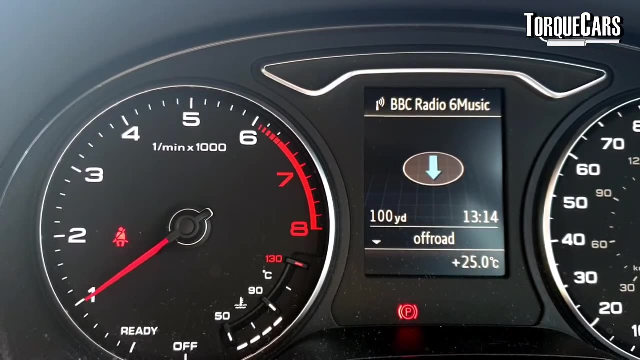 weekdays is a practical proposition. Most modern cars have actually got a trip computer on the dashboard that keeps track of your miles per gallon and that is a very useful tool. But often that's not accurate If you've added a piggyback tuning device or a tuning box. 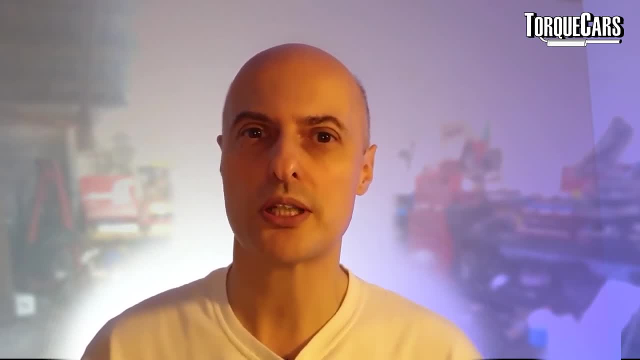 the car is often working from a false set of numbers, so it's usually underestimating the amount of fuel used. So this method to calculate your fuel is foolproof and it will work for every type of car and every type of vehicle. We're aiming particularly at our UK users because we 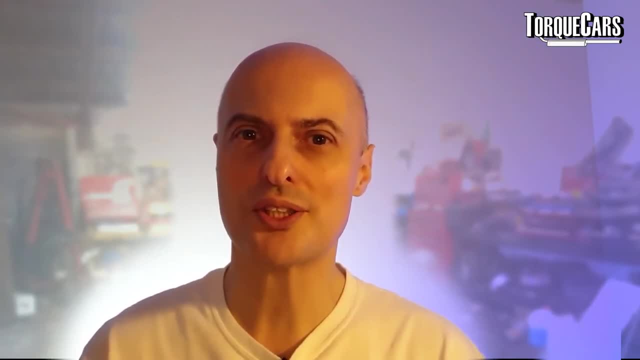 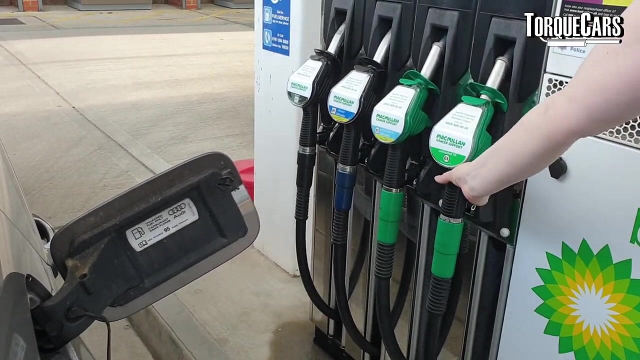 fill up in litres and not gallons, but in other regions of the world the principles still apply. So the first thing is you fill your car up to the brim. so when the fuel pump shuts off automatically, don't put more in, just accept that as your tank being completely full. That's your. 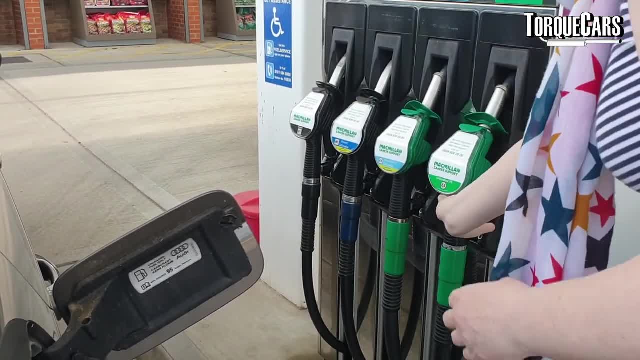 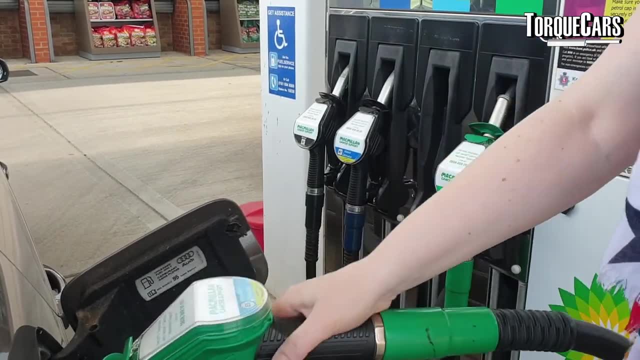 marker for next time, for when you come along to fill up again. Now reset the trip computer so your mileage is showing zero and just drive around on that tank of fuel. and the more fuel you use, the more accurate this will be. So make sure you get down to zero and just drive around on that tank of. 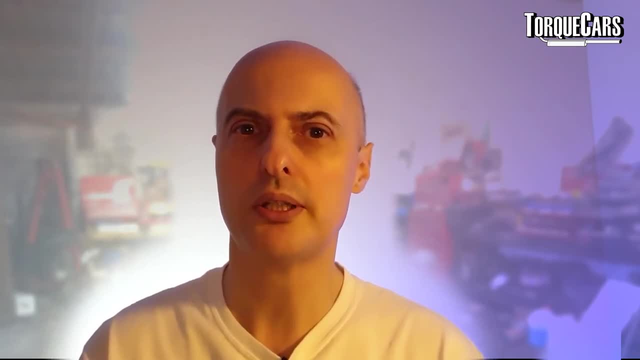 fuel, and the more fuel you use, the more accurate this will be. So make sure you get down to zero, to the red region, and fill up the car again, but note the amount of miles you've travelled and record the number of litres of fuel that you've put into your car. Now you've got the essential. 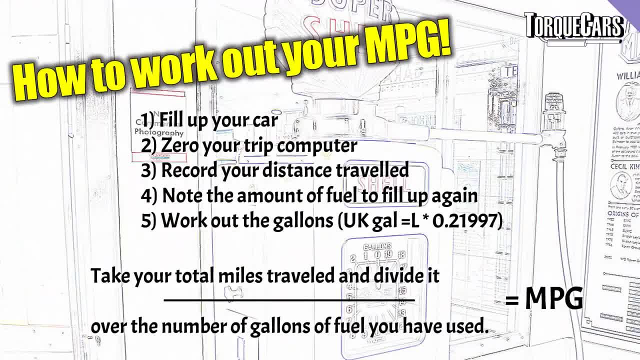 components to calculate your mpg. so you need to convert the amount of litres into gallons. That's done simply by multiplying by 0.21997 and that'll give you the number of gallons you've got. You take the miles you've driven, you divide it by the number of 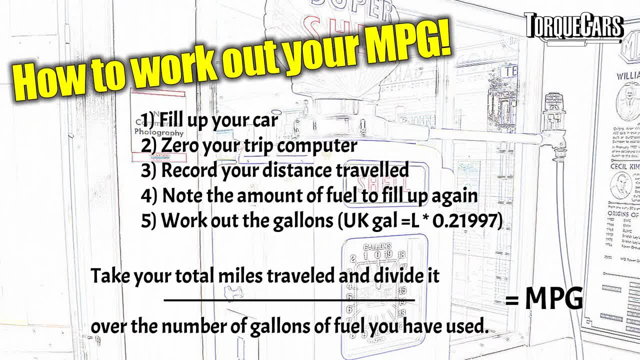 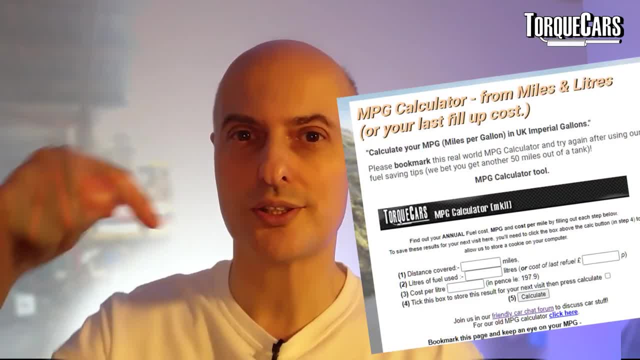 gallons of fuel you've used and you've got your miles per gallon figure. So what's the easy way of calculating your mpg? Well, we've got a calculator on our site. there's a link below in the description, if you want to follow that and it'll actually remember your last few fill-ups.